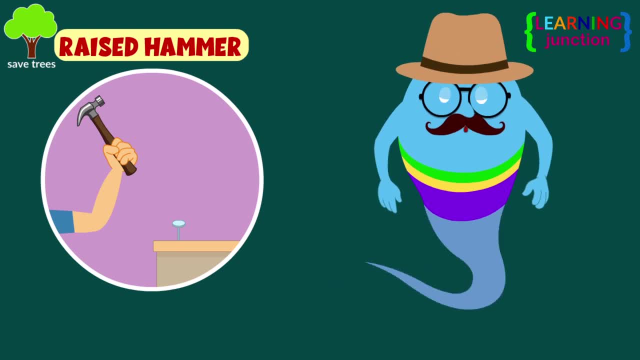 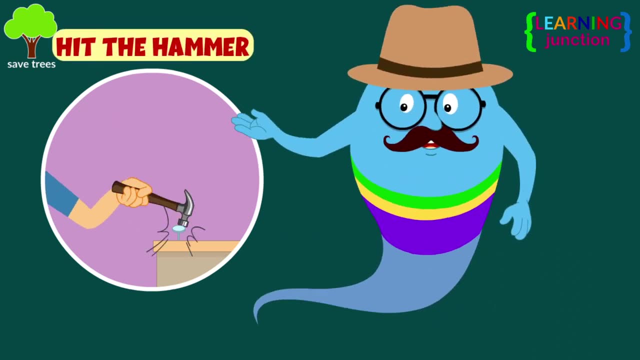 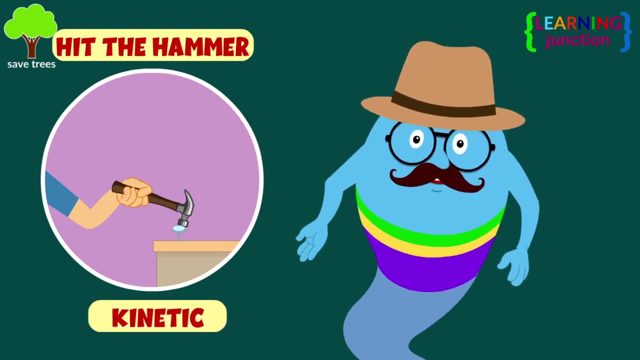 three things. First, the raised hammer has more potential energy, since it has the potential to go higher or lower. Second, when you hit the hammer on the table, the stored potential energy is changed to kinetic energy as the hammer is falling. Third, as soon as the hammer hits the table, the energy changes. 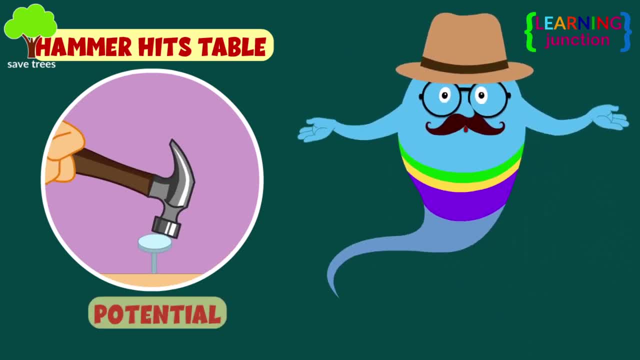 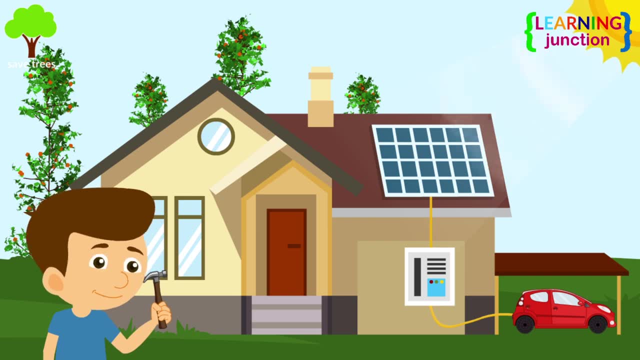 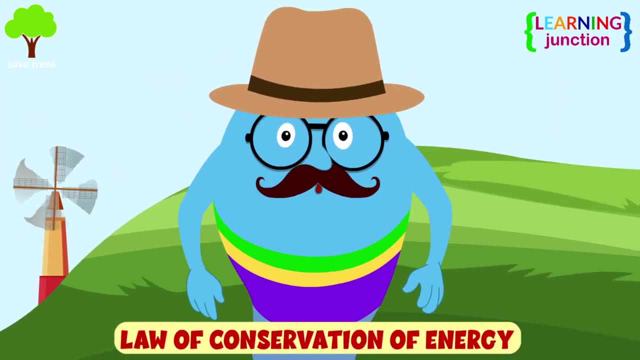 its form. The stationary hammer, then, has stored energy in the form of potential energy. You have seen that energy is neither destroyed nor lost during the whole task. It's only altered. It's only altered from one form to another, providing the law of conservation of energy. 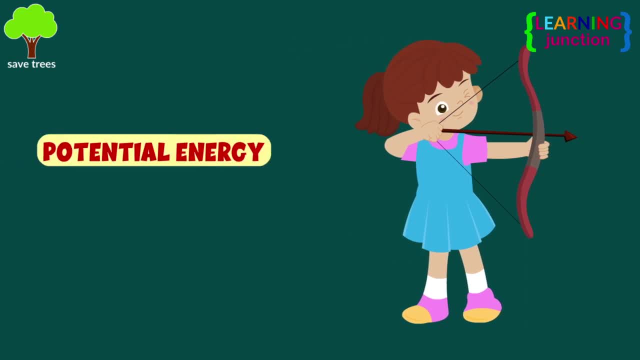 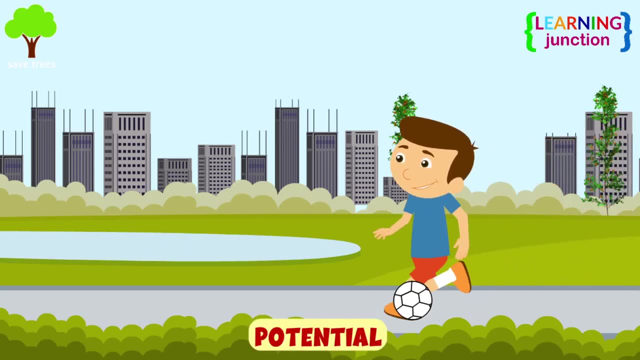 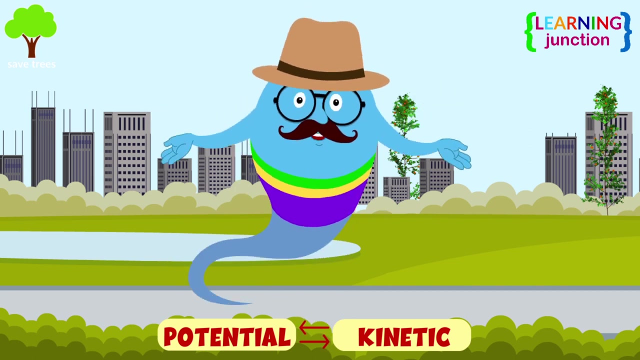 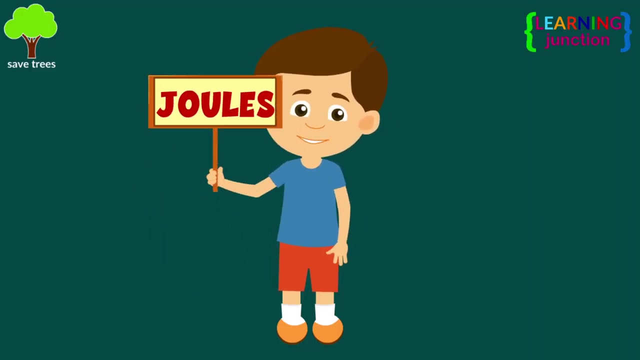 So you can say that potential energy is position- relative- and kinetic energy is motion- relative Potential energy transforms into kinetic energy and kinetic energy converts into potential energy, and then back again. It's a never-ending cycle. Look carefully, Both are measured in joules. 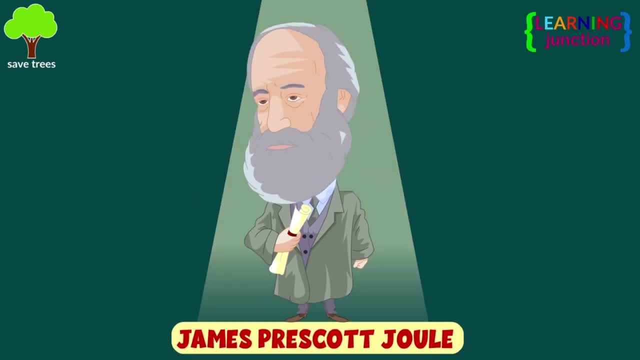 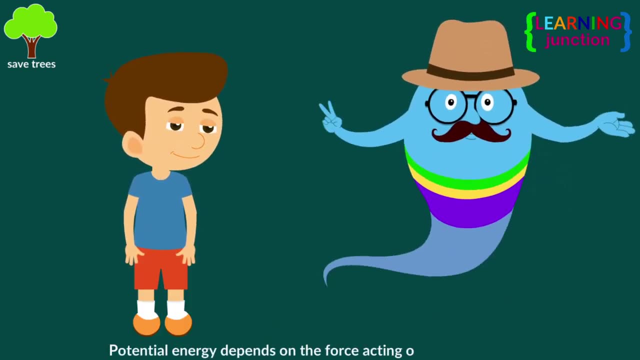 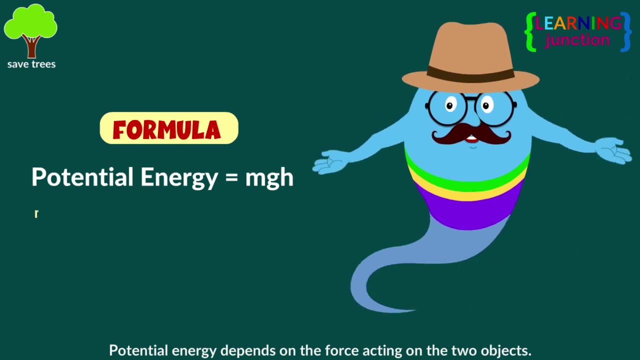 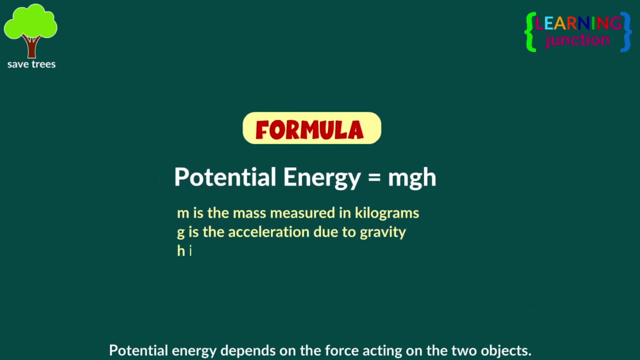 named after the English mathematician James Prescott Joule, born in Salford, Lancashire. Potential energy depends on the force acting on the two objects. Formula is: potential energy equals mgh. m is the mass measured in kilograms, g is the acceleration due to gravity, h is the 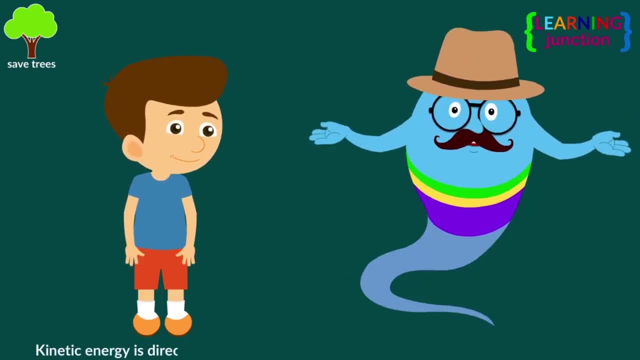 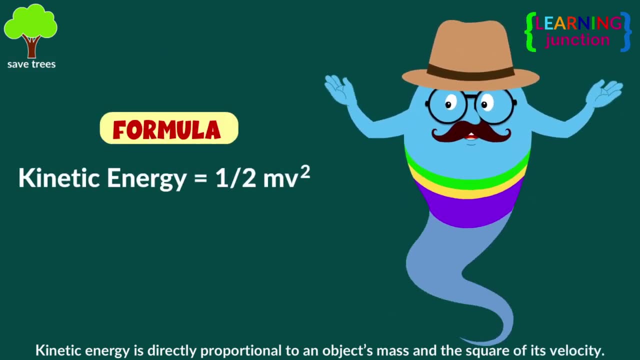 height in meters. Kinetic energy is directly proportional to kinetic energy. It's the same to an object's mass and the square of its velocity. Formula is: kinetic energy equals 1 half mv to the second. m is the mass measured in kilograms. v is the velocity of meters per second. 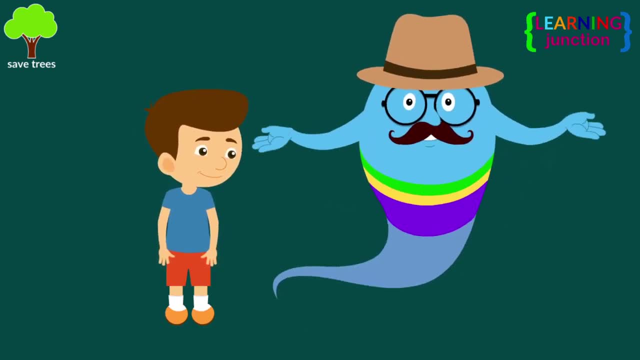 Now you know a lot about the potential and kinetic energy. Stay tuned for more videos. Bye-bye.